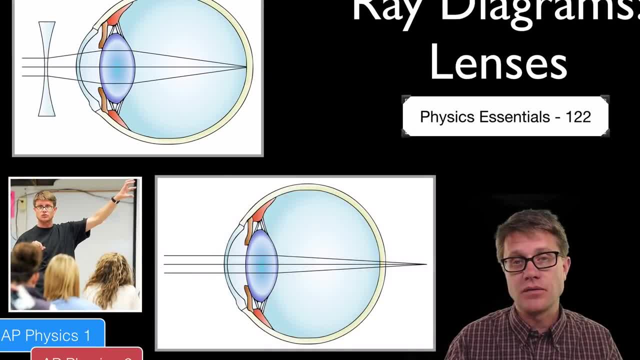 in the proper location, But you might be farsighted. If you are farsighted, you are putting the image too far inside your retina, And so how would we solve that problem? Just with another converging lens So we can focus it right at this point, back here, And so, when you are, 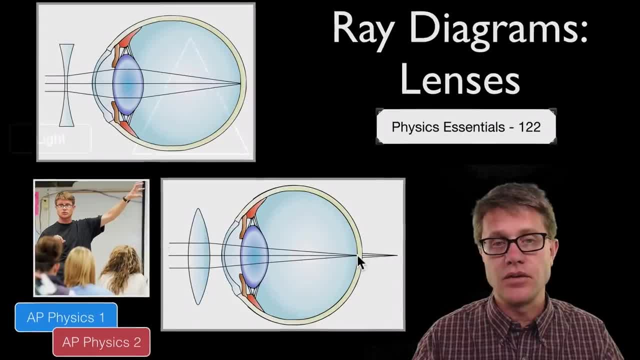 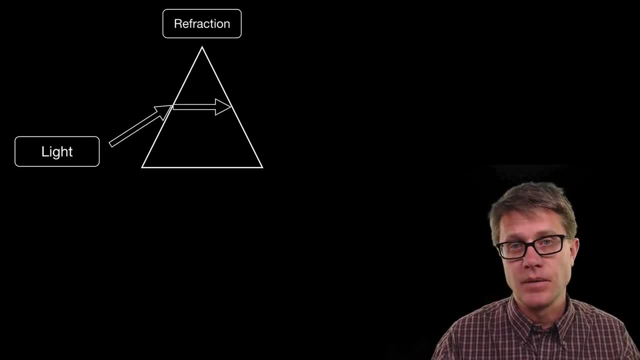 looking at where the image is created. remember, we are looking at the focusing of those rays, And so, light, as it moves from one medium to another, it can be bent. We call that a refraction, And what is doing the bending is going to be a lens, The ones that we will 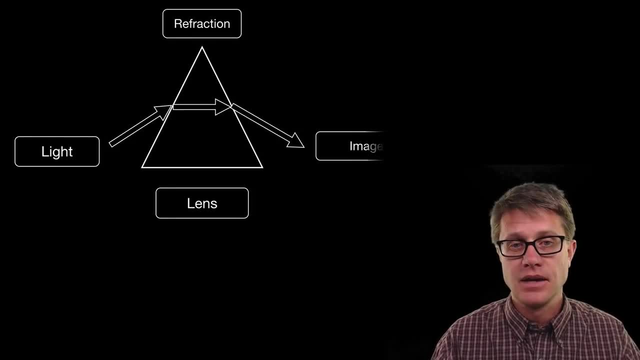 deal with in here are converging and diverging lenses made of glass, And so, as it does that, it creates an image. Sometimes that image is real And sometimes it is a virtual image. How do you tell the difference between the two? If you put a piece of paper there, the 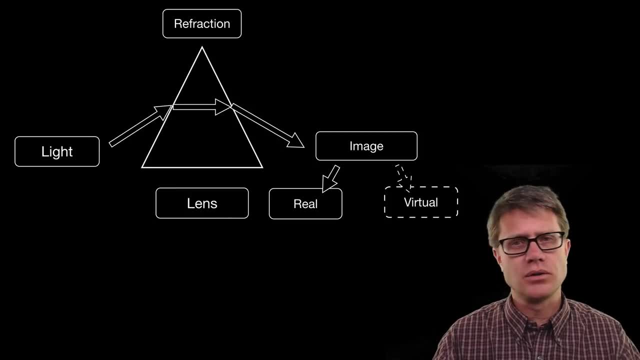 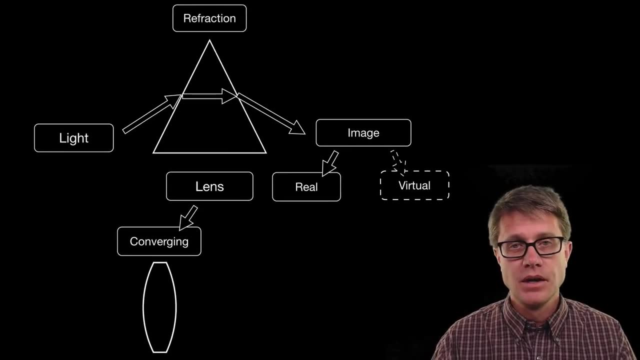 real image will show up and a virtual image will not. When you are looking at a mirror, for example, there is a virtual image of you on the other side, But you cannot put a piece of paper there. You simply cannot get in. Lenses we will deal with are going to be converging and diverging lenses And a way to figure. 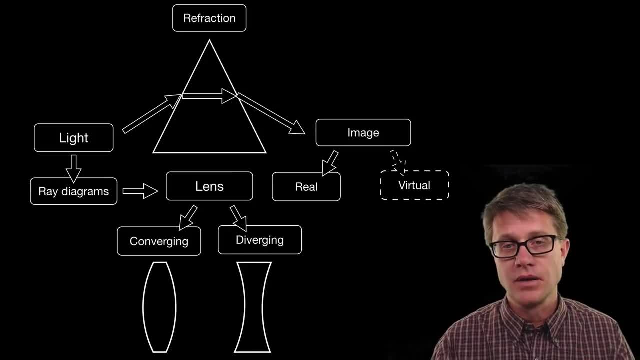 out where that image actually is is to use a ray diagram. We will draw just two or three rays in each of our drawings, So as the rays come in, they will either be converged or diverged, And figuring out where they go tells us where the image is going to be Before we get to. 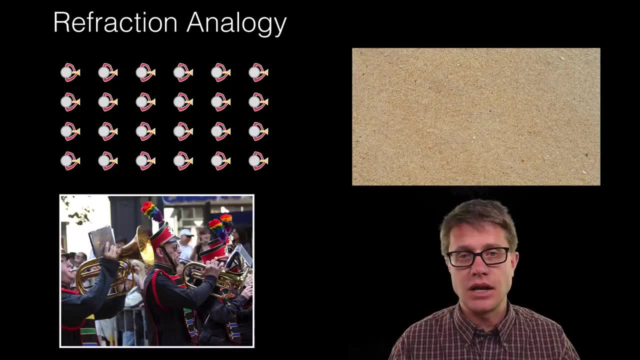 that you should have a good gut feeling for how refraction occurs, And I use a marching band analogy for this. Imagine a marching band is going down through a parking lot. They are keeping. we are looking at it from above And they are keeping, we are looking. 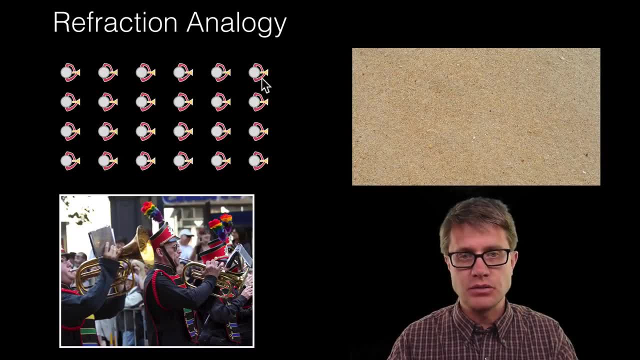 at it from above And they are keeping. we are looking at it from above And they are keeping. we are looking at it from above, But each of the trumpet players keep an equal distance between them and the person next to them, And so, as they are marching through, 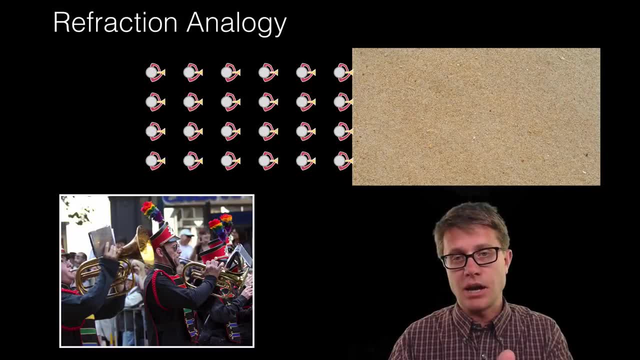 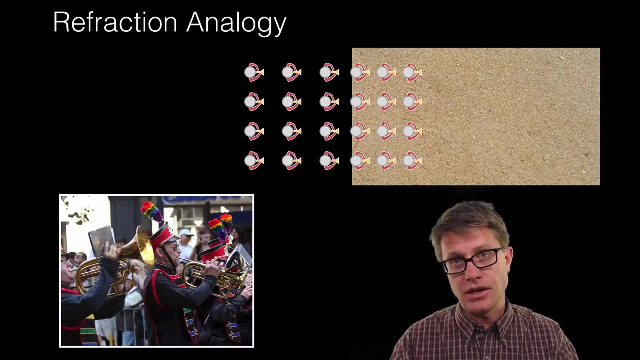 the parking lot, they eventually come up to some sand, And so what is going to happen to that group in the front? Well, it is going to slow down compared to the ones behind it, But since there is no angle here, it is simply going to go at a slower rate through it, and 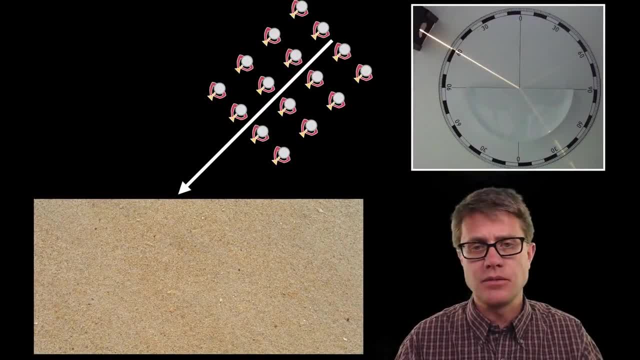 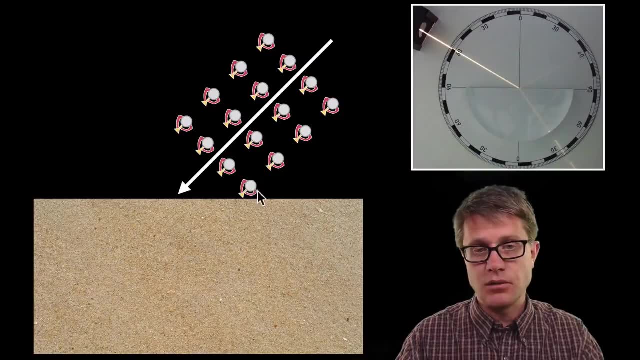 there would be no bending or no refraction. But watch what happens if we come in at an angle like this. As it comes in at an angle, which of those trumpet players are going to slow down first? It is going to be the one on the bottom, And so, as the one on the bottom slows down first, 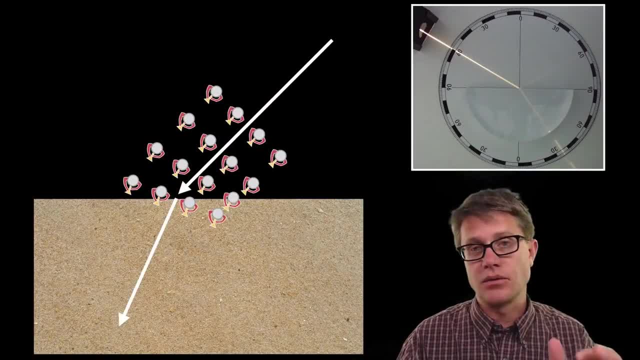 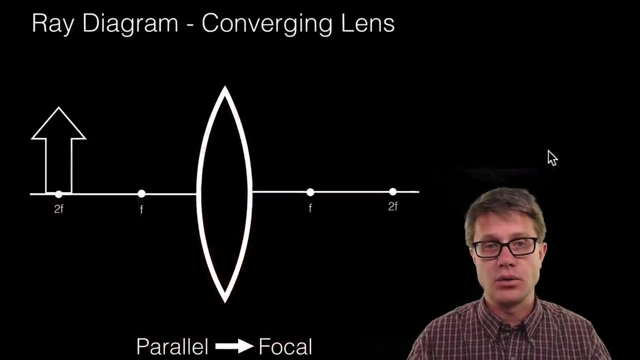 watch what happens to the other ones. They are bending like that. So we get refraction And you can see that right here. As the light comes in, as it hits the glass, it is refracting here because it is traveling at a slower rate. So let's get to a converging lens and figure. 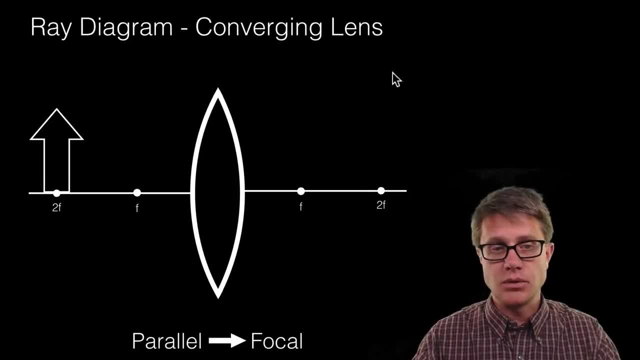 out where that image is actually going to be. Now there are a few things we want to define. We first got 2F and F. This stands for the focal point And this is two times the focal point For dealing with mirrors. we sometimes call this the center of curvature, So you can imagine. 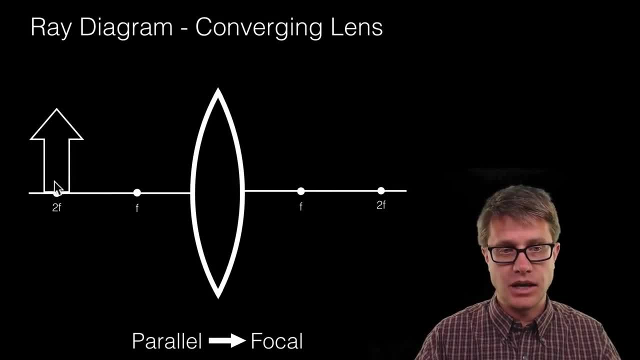 if this is a circle over here, the radius would always be the same: 2,, 2F right here. So let's draw how this works with a lens. Again, the light is going to go through this lens. This is glass and this is going to be air out here. So to draw that, you first start. 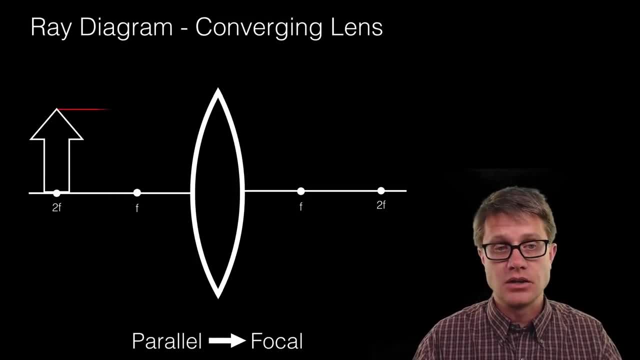 by taking the top of your image or the object rather, and you are going to draw a parallel line into the lens itself. So we are going from parallel and then we are going to go through the focal point, So we are going to draw a parallel line into the lens itself. 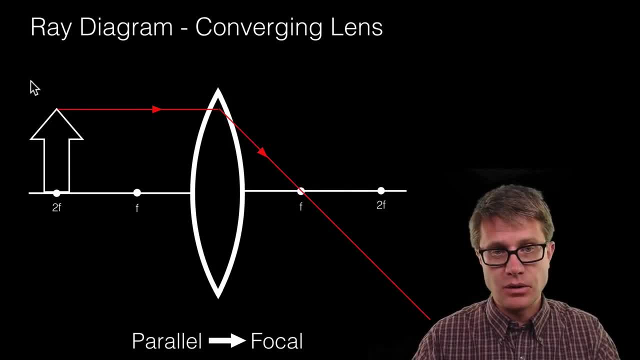 And so we draw a line like that, And so that is going to bend or refract right here and it goes right through the focal point, like that. Now let's turn that around and we are going to start by drawing it through the focal point. So how do we do that? We draw a line. 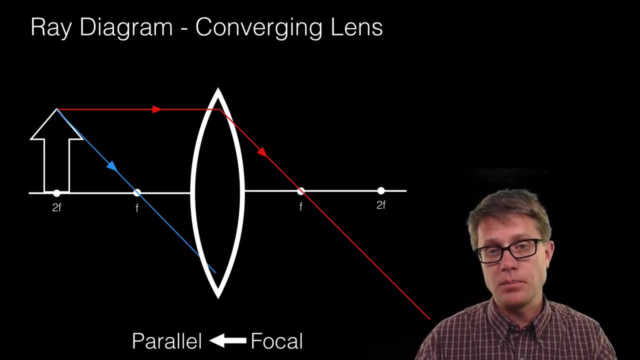 like that. So now we go through the focal point and now it is going to go parallel, And so now we have got converging- you can see the converging rays over here. And so since those rays are converging, we know that the image is going to be upside down here. 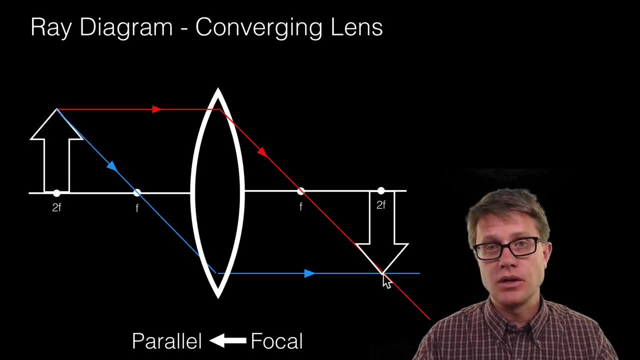 So this was the top over here, And we also know that it is going to be a real image, a true image, In other words, you could put a piece of paper right here and you would have that on the other side, Just like you have a true image on the inside of your eye. 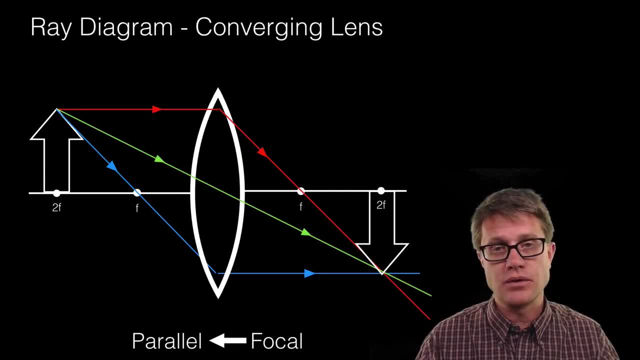 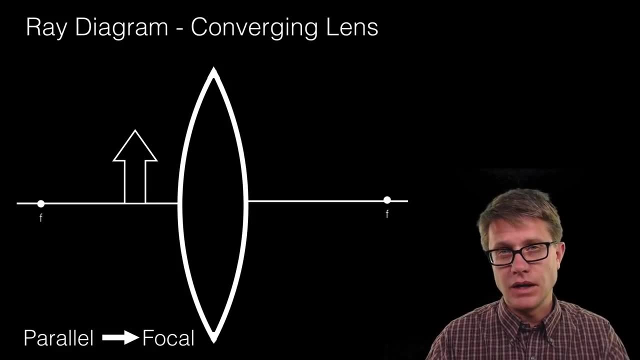 Now we can check ourselves on this as well, So you can draw another ray that goes right through the center of the lens, And so we know that this is going to be where that image is going to be. Now let's watch what happens as we move inside the focal point, It gets. 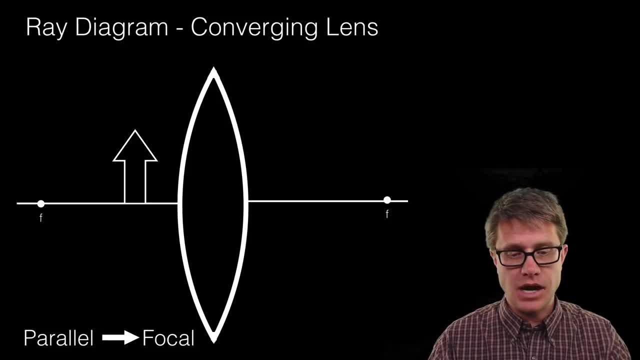 a little bit of weird here. And so what do we do? Again, we draw from the top of this object here, We draw it parallel, And then we are going to go through the focal point. But now it is a little bit different, since we are inside the focal point. How do you? 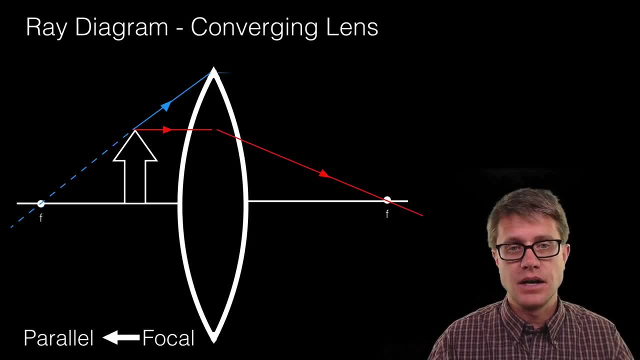 draw it from the focal point. Well, it is going to look like that, And now it is going to be parallel, like this. And so, as we look at this, these two rays on this side are diverging from each other. You can see that they are not going to intersect at any point, And so 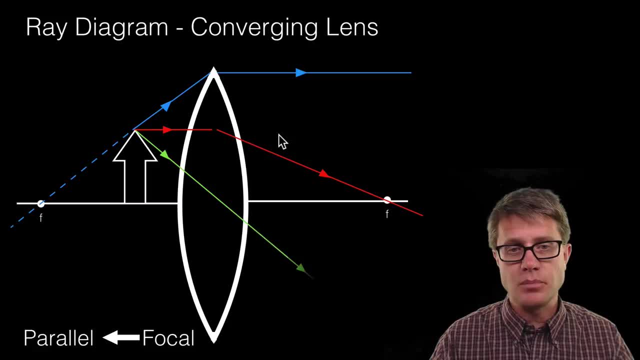 we are not going to find an image on the right side, We are going to have to play those backwards. Same thing with the line through the center. All of these are diverging, And so we have to play those lines backwards. And so where is our image going to be? It is going to be. 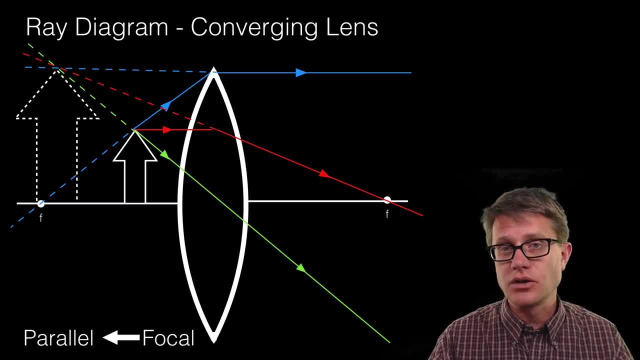 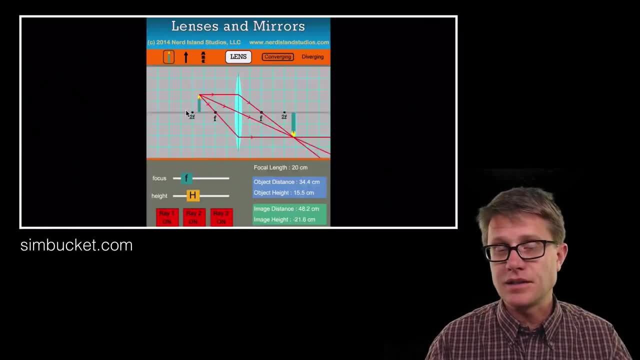 on the same side as the object. We now call this a virtual image. You could put a piece of paper there and it is simply not going to show up. But that is where it is going to appear to show up. Now let's test this. So we are going to use a Simbucket simulation. 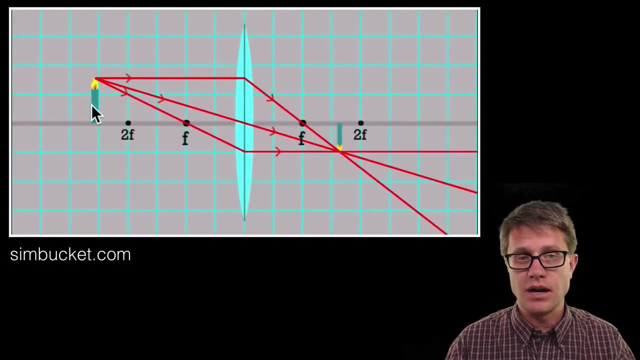 So we are going to be able to drag the object on the left side And you can see as we drag the object. the image is true and it is on the right side, But watch what happens as we approach the focal length. Now the image is on the left side And it is going to be a virtual image. You can see. 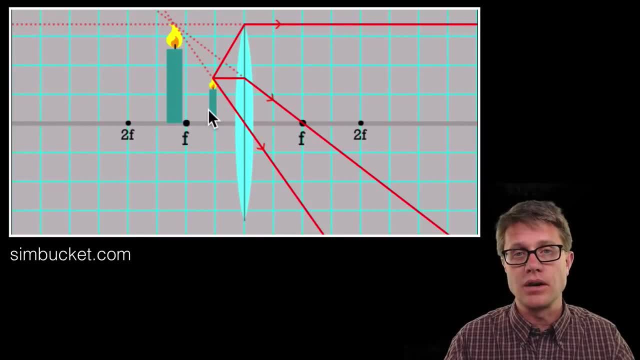 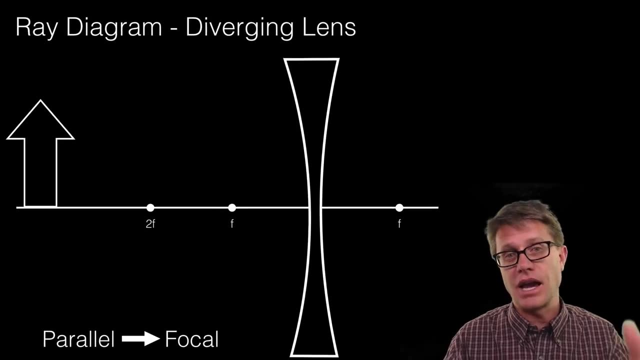 that through the dotted lines right here, And we can even measure the distances to figure out where that image is going to be. A better way to do this is actually use lenses and figure out where those objects are going to be found and the virtual or true images. Now 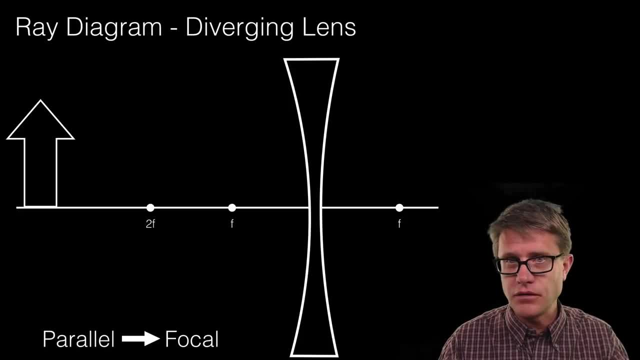 let's go to a diverging lens. And so how do we do this? Still have a focal point, Still have 2F. I start by drawing that parallel And then we want to draw through the focal point. That is the tendency. 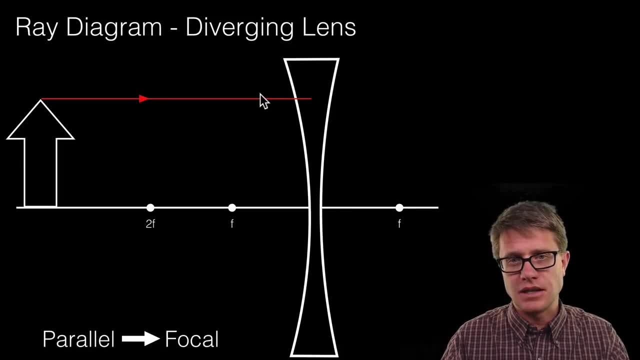 To draw it right down in this direction. But remember, a diverging lens is not going to do that. If a marching band is approaching, it is going to bend away, and then bend away like that. And so what focal point are we going to use? We are going to use this focal. 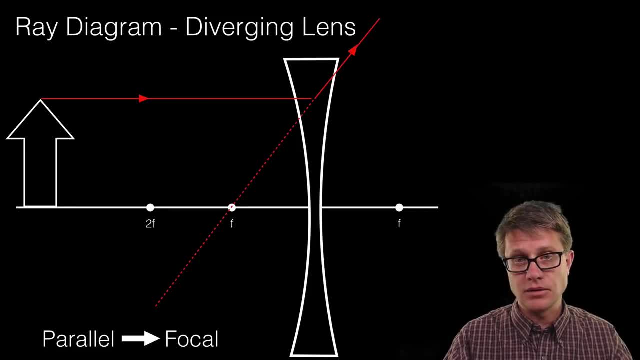 point right here. So that is going to be where the ray moves out. And now we could go through the focal point. So it goes like that: Where is going to be our parallel line? It is going to be like that. And so on the right side again we have all these diverging lines back.